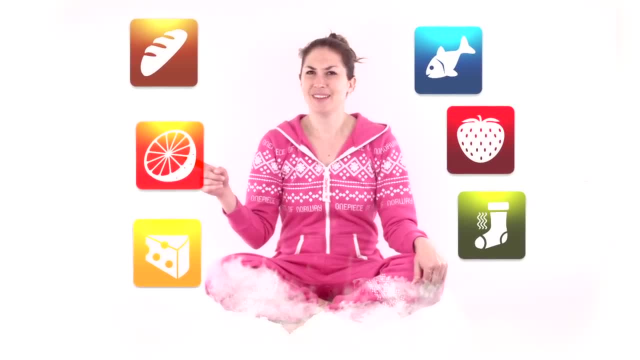 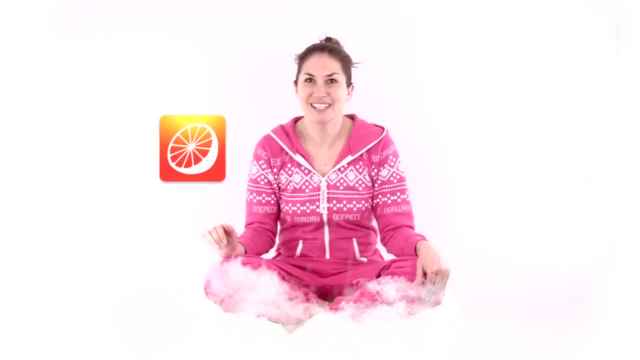 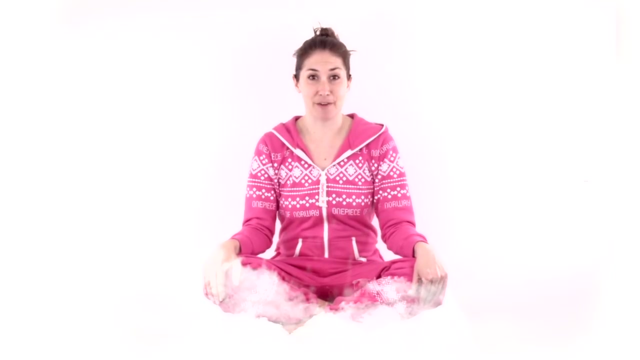 That's tempting, Oh, but look, Let's smell the orange. Oh, it's so good, It makes my mouth water, Yummy, Mmm. Now, sometimes it can be tough to just focus on one thing. There are so many other things that we get distracted by. If 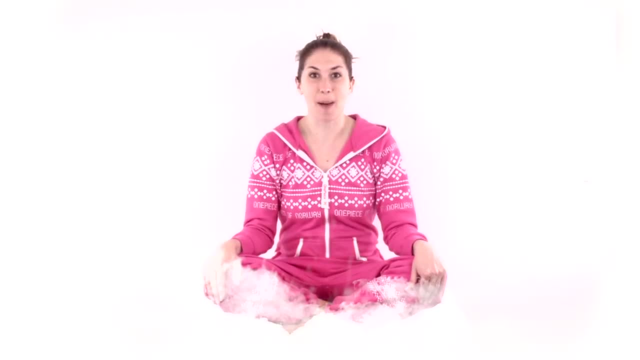 we practice, though, we can get really good at being focused. It means we can learn more and become really skilful at doing stuff, which is great. Sometimes it's called concentration: We concentrate on something. Now, we all need to practice this, even our mums and dads too. Hmm, Let's have a go now, shall we Ready? Okay, let's. 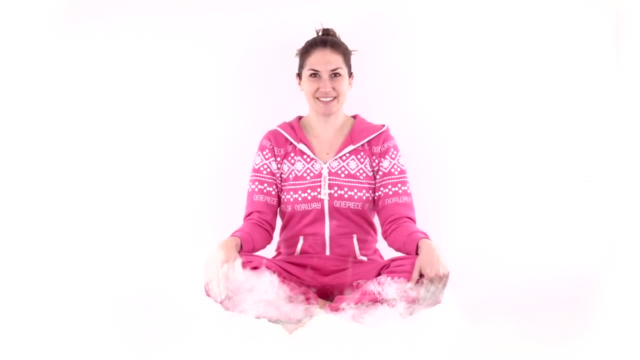 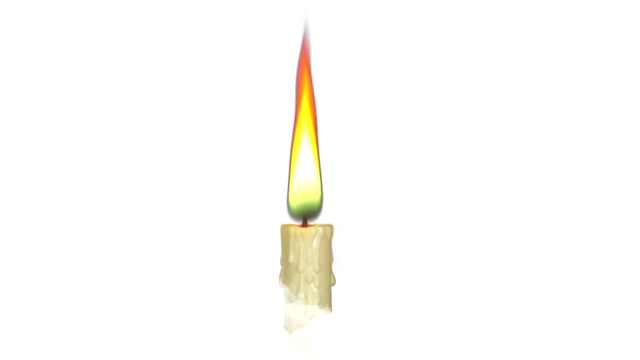 get ready. We sit nice and still eyes open and looking at me. Can you see that The candle flame? Wow, Let's look very carefully at it. We watch its tip moving and flickering around. We see the different colours inside it: The yellows, the orange, a little green. 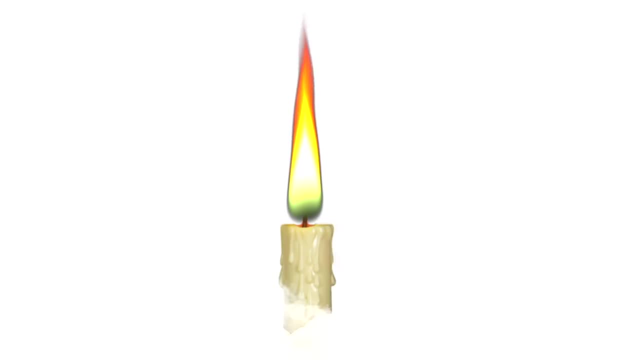 maybe the bright light. Can you see them all? Yes, We keep looking straight at it, focusing our whole mind on it, filling our mind as we concentrate on it. Look, now we try a special trick, some real magic. Keep looking at the flame. After I count to three, let's close our eyes and 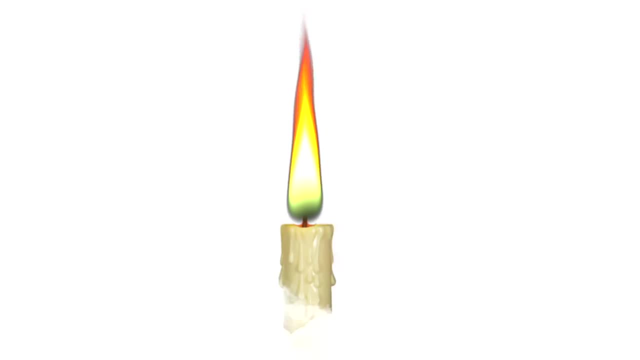 see if we can still see the flame even with our eyes closed. Ready, One, two, three, Close your eyes. Can you still see it? You can still see the flame in your mind even though your eyes are closed, But it might be fading away. That's fine, Just open.